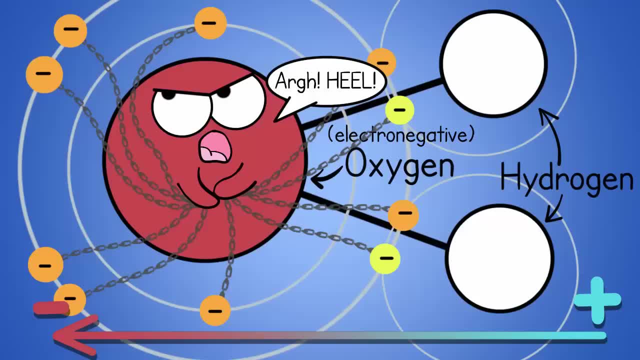 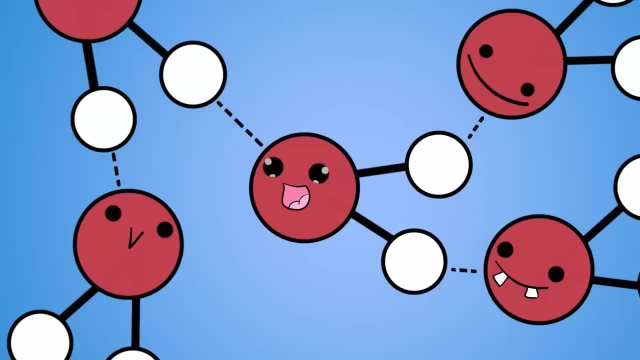 because of the electrons that are spending more time next to it, And it gives the hydrogens a slightly positive charge. Well, that means that other water molecules have an easy time bonding together, Why? Well, because the hydrogen of one water molecule, with its slightly positive charge, 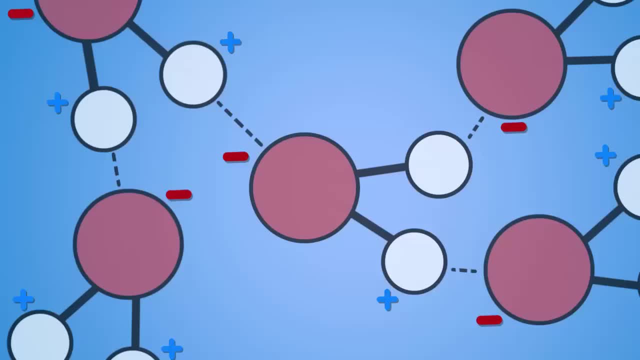 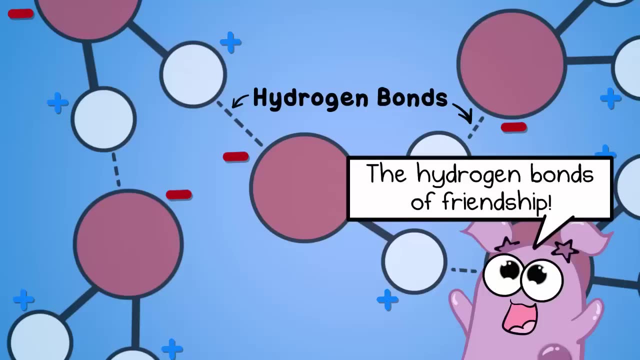 can bond to another water molecule's oxygen- with that slightly negative charge. So the hydrogen bonds among the water molecules are hydrogen bonds, And these are the very bonds that allow water to have many of the properties that we're about to talk about. Have you ever? 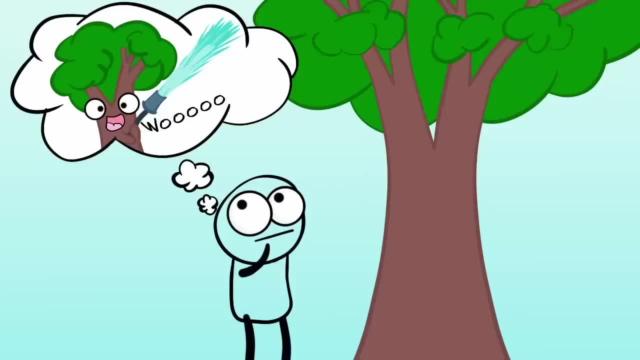 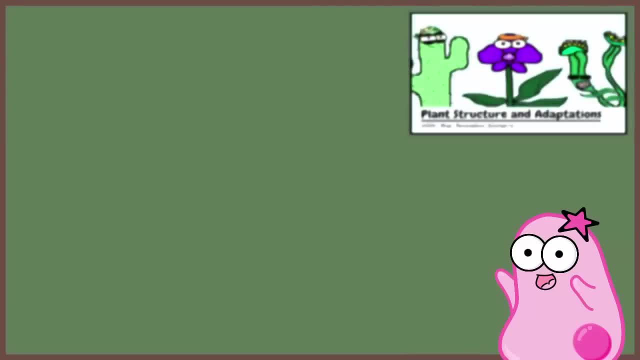 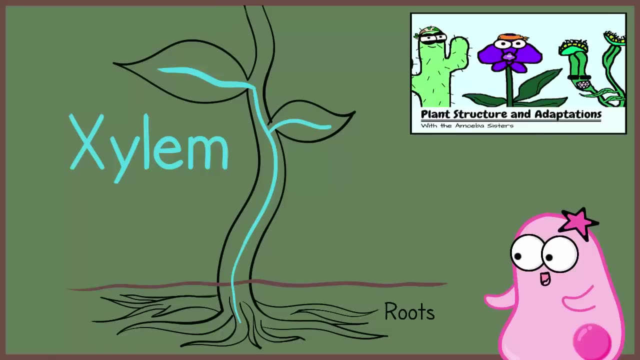 looked at a really tall tree and wondered: how does the water get all the way up there? I mean it's got to go against gravity, Gravity. Well, in our plant video we talk about the xylem. It's vessels within certain types of plants like trees, and these vessels transport water. 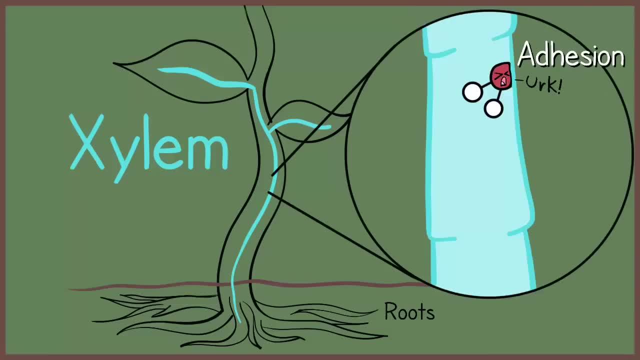 But what's really neat about water is that it's not just a plant. It's a plant. that's water is that it sticks to the xylem walls in what is known as adhesion, And this helps fight gravity. But water molecules- with their hydrogen bonding, they also bond to each other in something. 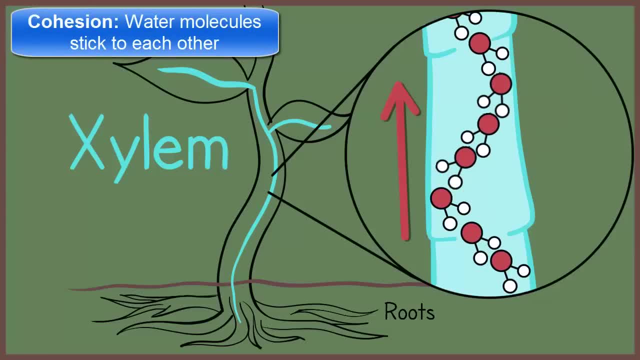 called cohesion. It's almost a beads on a string kind of fashion. Water molecules evaporate from a leaf and then the next water molecule in line is pulled up upwards, and so on. This cohesion is really a big deal. Cohesion is all about cohesion. It's all about cohesion, It's all about cohesion. 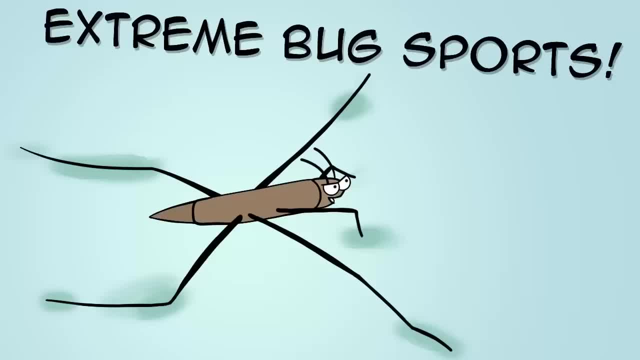 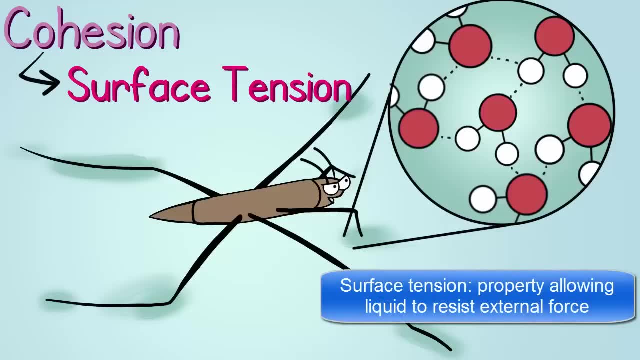 It's also a reason that water striders, one of our favorite insect types, can skate on water. Cohesion contributes to the surface tension of water. Water actually has quite a bit of surface tension compared to many other liquids, And it's not just water striders that can walk. 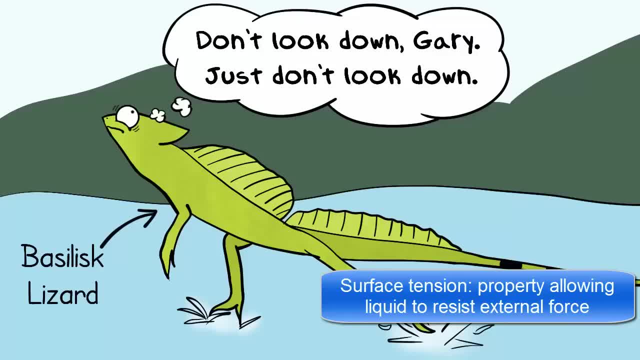 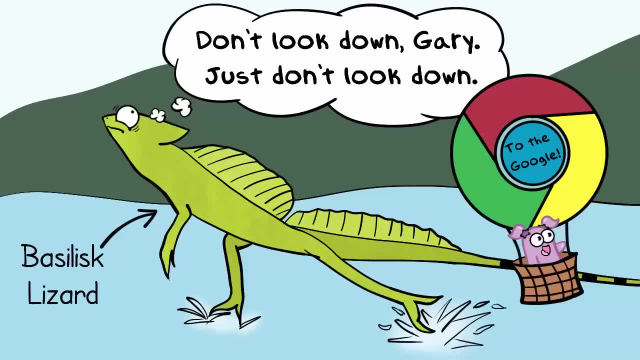 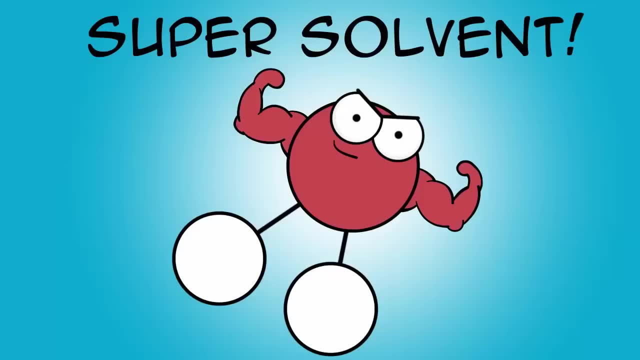 on water. There are a lot of insects, spiders and even larger animals like reptiles and some birds that have the ability to walk on water. So to the Google for that. So water is a very powerful solvent for other molecules And that means that water can dissolve many other. 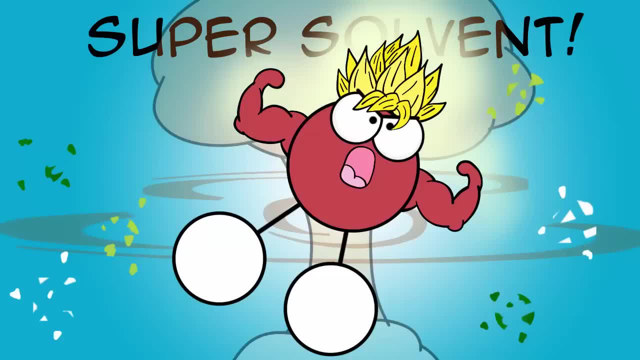 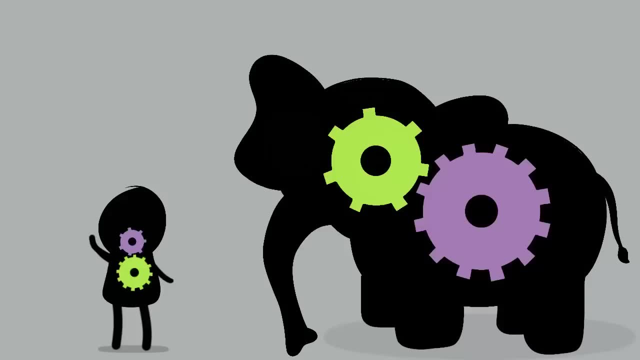 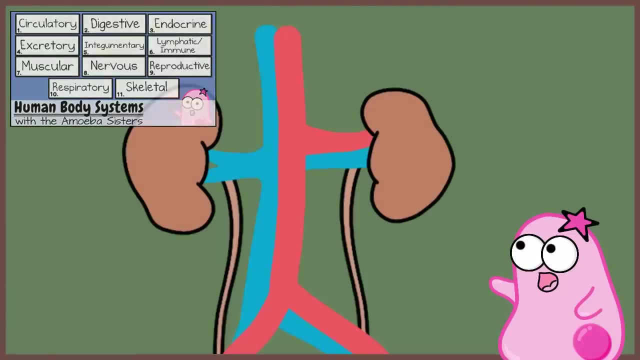 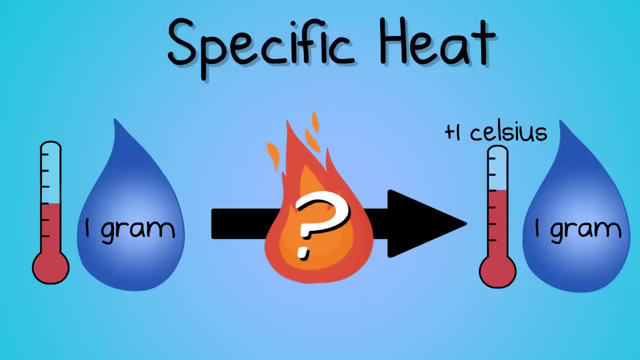 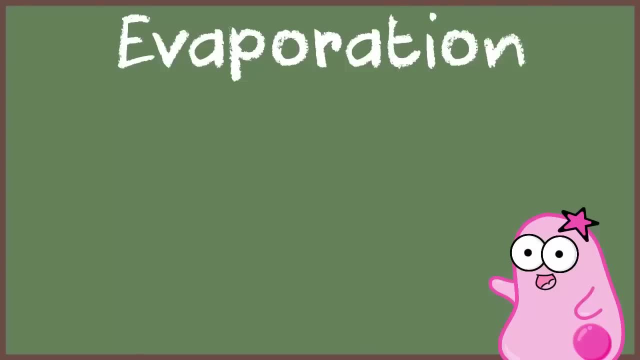 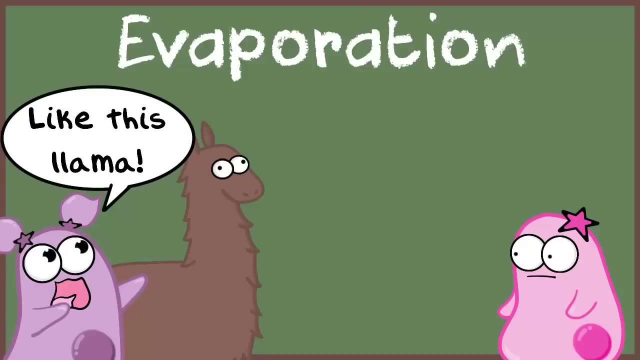 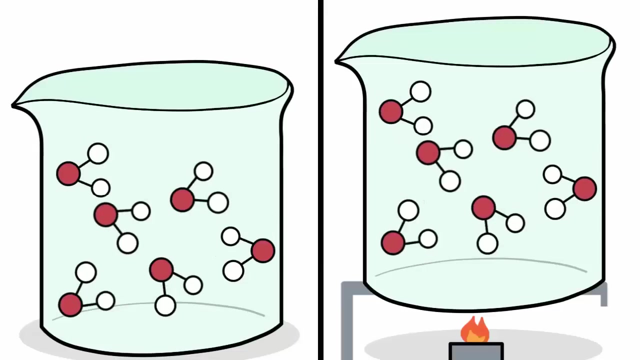 This also impacts the environment. Now, still on the topic of temperature, consider evaporation. Many animals rely on evaporation to cool them. Think of water molecules. They are moving, but those that have more heat energy, they're moving the fastest. 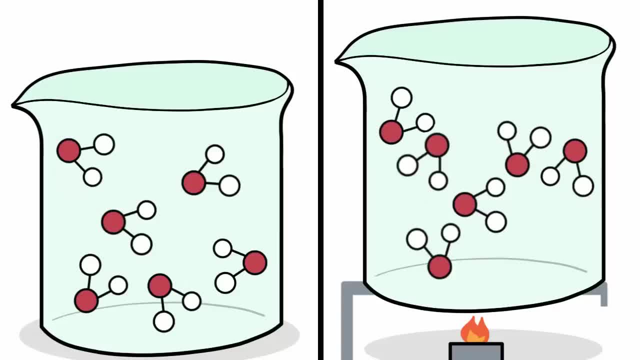 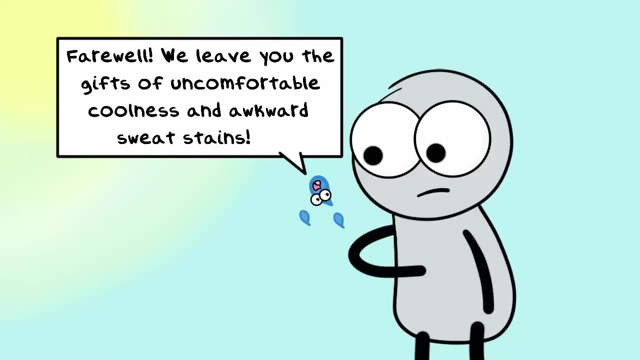 And they're the more likely molecules to make the phase change to gas. And these molecules, as they leave their energy, their heat, is no longer on your skin. And, by the way, all of this is not just animals too.